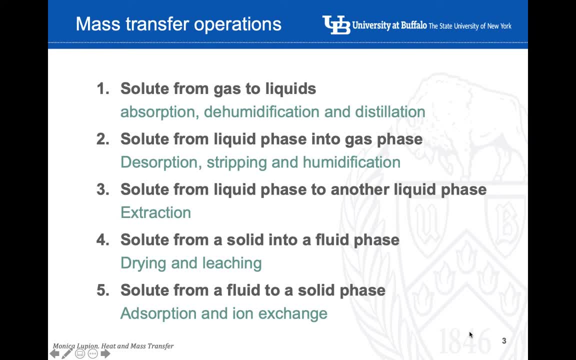 we can define absorption process, dehumidification and distillation. Distillation, for example, is a combination as well of energy balance, because we will separate the different components of a mixture in relation to the boiling point. So we need to put energy into account as well. 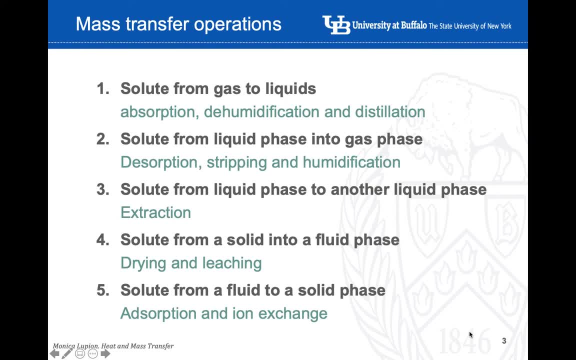 Okay When we want to separate an element A from liquid phase into gas phase- that is the way around, the other way around- then we call the operations like adsorption, which is the same as stripping and humidification. If we have two liquid phases and we want to transfer the solute from one liquid to another. 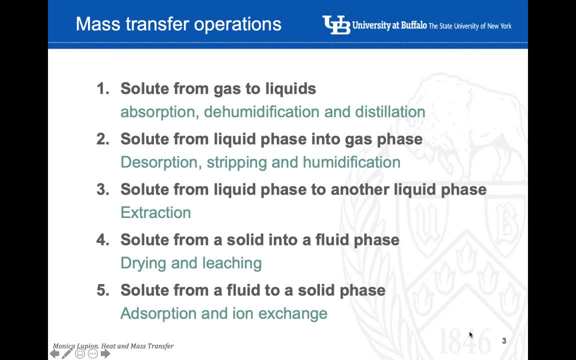 this is a typical example of liquid-liquid extraction. What about between solid and gas or liquid phase? Well, if we want to transfer the solute from a solid into a fluid phase in general, then we call it drying and leaching. Otherwise, the other way around, the opposite process. if we want to transfer 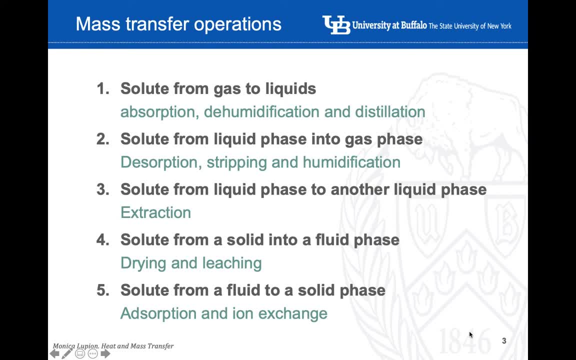 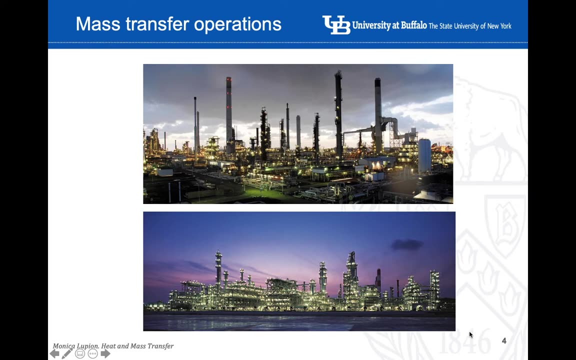 a solid, from a fluid phase to a solid phase. then we call it adsorption with D and ion exchange. This is a picture. these are two pictures of different processes in industry, most likely a refinery, And you see all the towers here. they are most probably mass transfer equipment. 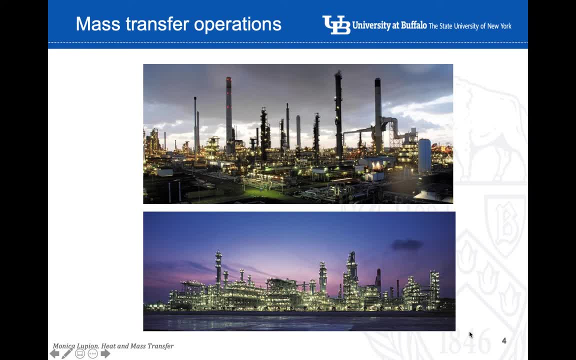 either a gas or a solid. These are either absorption units or desorption units or distillation columns, because they're usually very, very tall. But in addition to that, I'm pretty sure that you'll find different elements here, different equipment, operating mass transfer, the same as heat transfer. 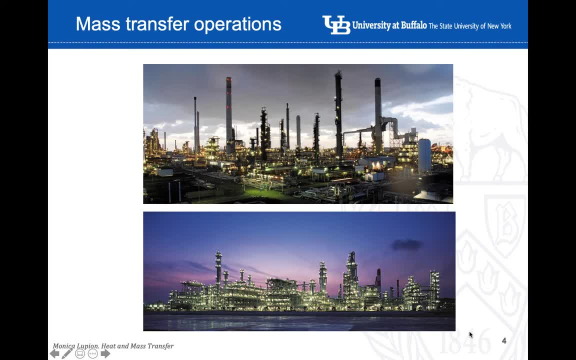 They are very, very common in industry. Those are probably the two main pillars of any chemical process when we need to transfer some elements from one phase to another Or if we want to increase the heat of any particular stream for some reason. So heat transfer and mass transfer are really really very common in industry. 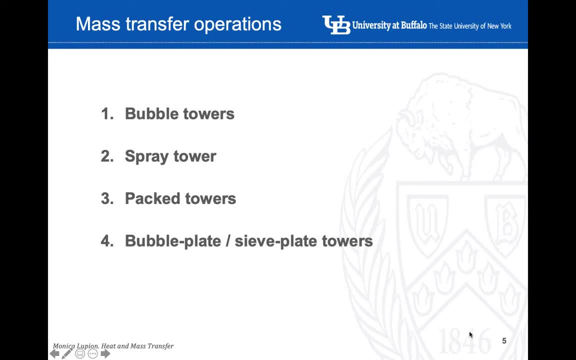 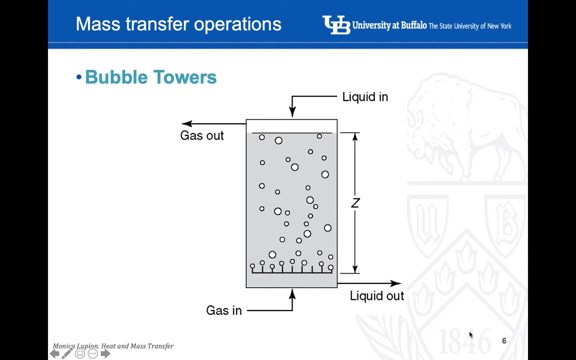 Let's see together a few examples of mass transfer equipment, And we're going to see four different examples: Bubble towels, spray tower, packed towers and C plates towers. The first, the first example, is a bubble towel. What we have here is just a. 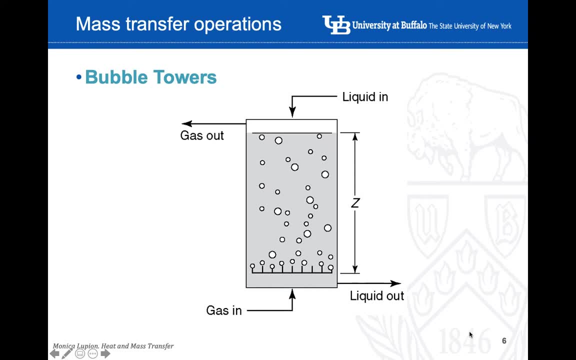 tank filled with liquid and we inject gas with of course different concentration in the inlet as in the outlet. Important parameters here in the design of equipment is the height and the diameter as well, but most critical is the diameter of the bubbles. You see in the picture how we produce bubbles. 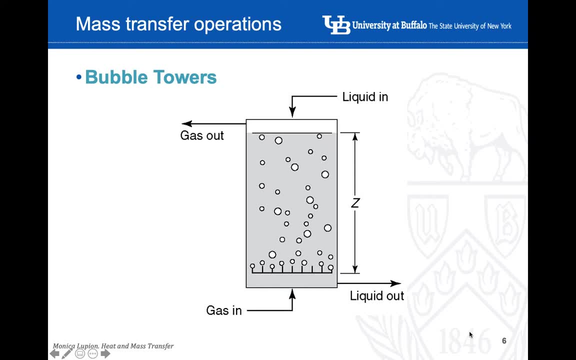 using some kind of device. Actually, this is critical for mass transfer operations in general. We need to achieve a very good contact between the phases. That's the only way that the mass transfer can happen. if there is an intimate contact between, in this case, the gas phase and the liquid phase, How? 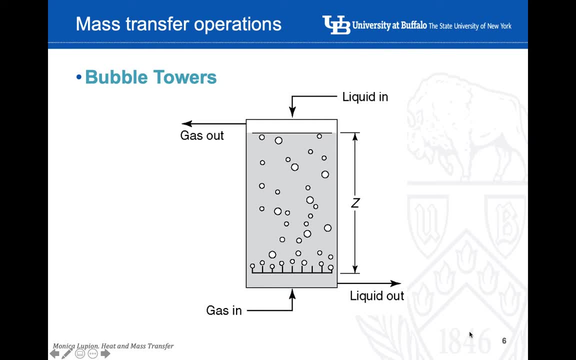 can we achieve that? Well, one way is to increase the contact surface, and we do that by producing a very small bubble where, let's say, the relative surface in relation to- you know, just putting- contact gas and liquid is higher, is improved and therefore we can achieve a very efficiency during the mass transfer operation. 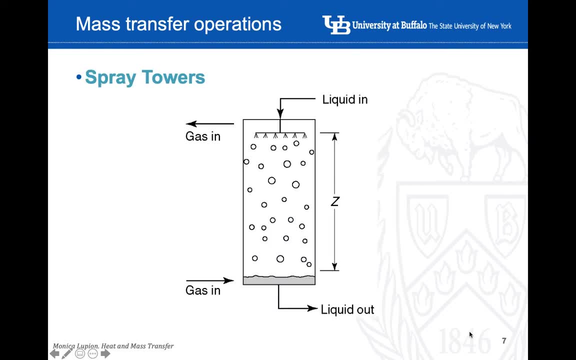 The next equipment is a spray tower, is just, let's say, a mirror of the previous process. In this case, what we do is a tank which is full filled with gas and we spray liquid. it's like a shower of a sprinkle, and with the same aim as in 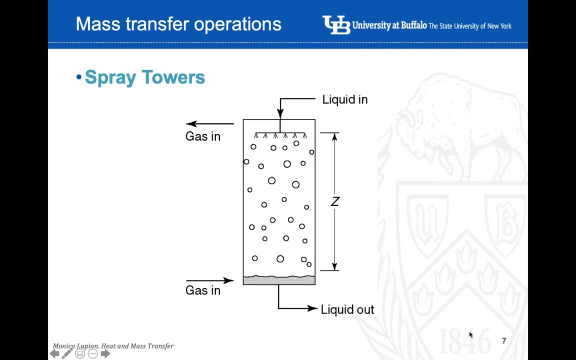 previous example. we need to have very tiny particles of liquid in order to have an improved contact surface in order for the mass transfer to happen in an efficient way. This is a very typical example of desulfurization process. Let's imagine that we have a boiler and we're burning any kind of biomass or coal and there 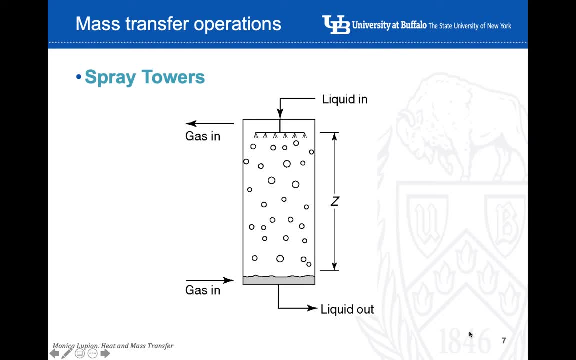 is a production of sulfur components, which are present in the flue gas. What we do here is to eliminate the sulfur components in order to meet environmental regulations, So the gas that is getting in will get into this spray tower with a higher concentration of sulfur. 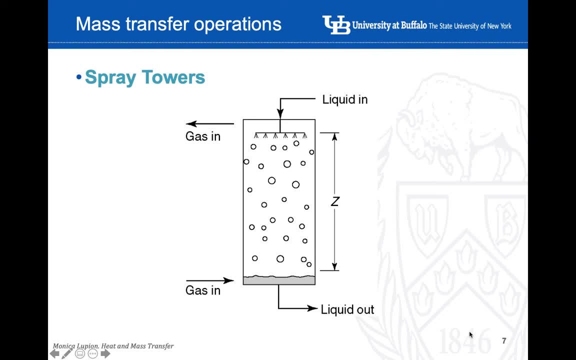 Then we spray in a counter flow. we spray some liquid with some formulation of chemicals that are desulfurized, So we spray the gas out of the spray tower, which has the capability of absorbing the sulfur components. as a result, The gas that is getting out is almost free from sulfur compounds. 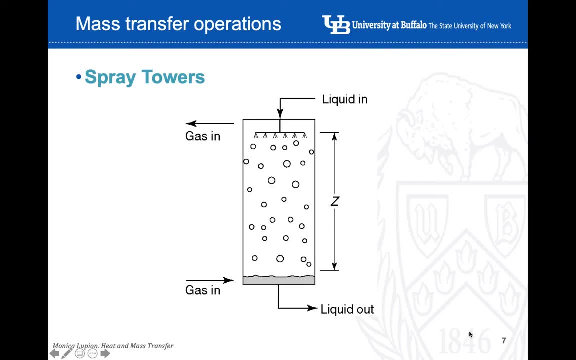 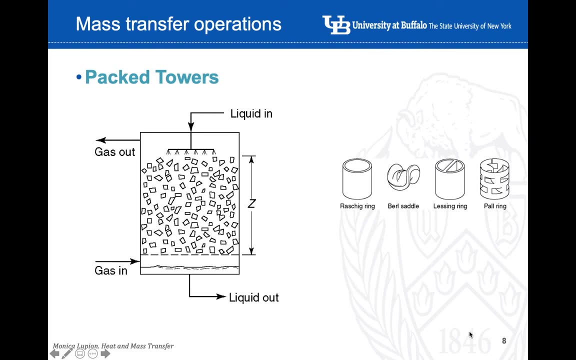 Then, of course, we need to treat the liquid that's getting out because it's loaded with sulfur compounds. Pact tower- this is another example of desulfurization. The composite is similar to what we've seen so far, So we put in contact. 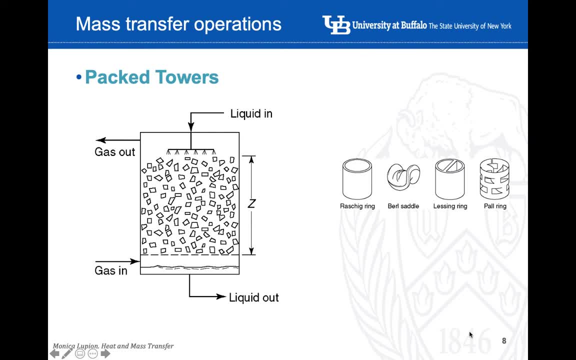 different phases and trying to optimize the surface area, trying to make the contact better between the phases. But on top of that, what we do here is to incorporate some elements inside of the tower. We do this to force the gas or the liquid that is getting in to follow a longer pathway. 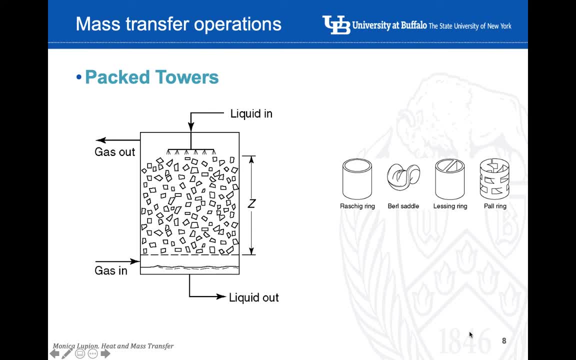 to increase the turbulence inside of the column or the tower. The reason why we do this is again to increase the contact, to improve, to make the contact more intimate between the different phases. If we increase the turbulence then we make the phases to have a better contact. 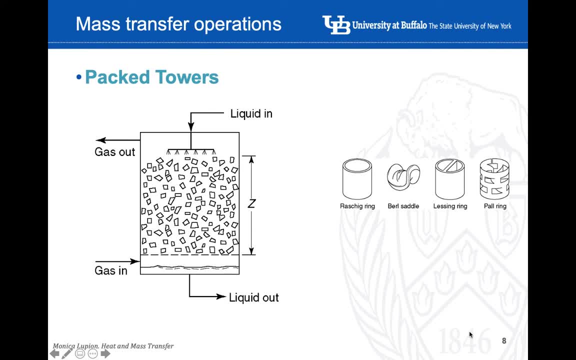 and therefore we can achieve a better and more efficient mass transfer operation. There are different ways to do this. There are different packing materials that we can use, depending as well of the type of liquid and the type of gas that we are using in the system. 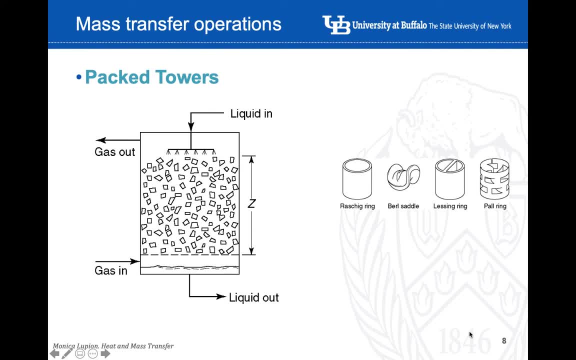 One thing that I should mention is that, well, the packed towers could be more efficient compared to a tower without any packing material, but the cons side is that we need to put more energy into the process To overcome the delta P, the pressure loss. 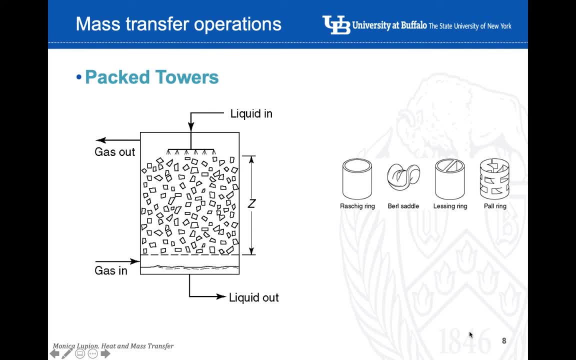 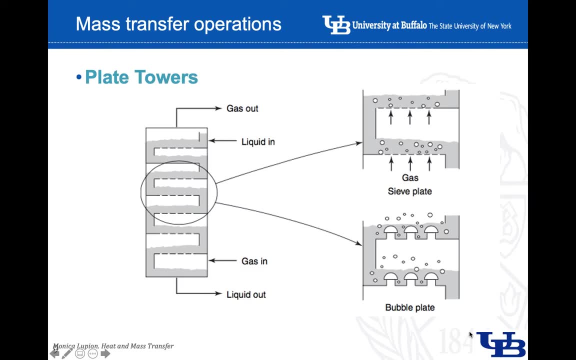 So you need to put more energy into the system for the gas and the liquid to go through this packed tower. The last example before we get into the particular case is the plate tower. In this case, what we have is a different trace. 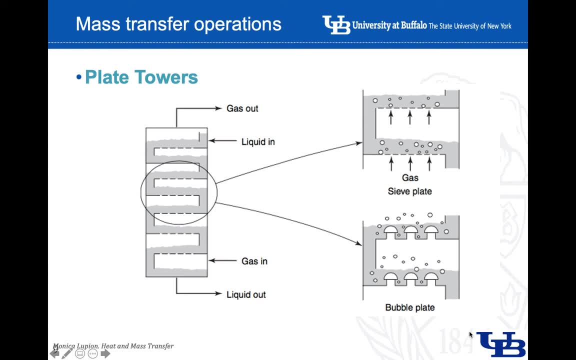 inside of the tower And in each of these trays there is equilibrium between the different phases: the gas phase and the liquid phase. We produce as well. well, these trays have some holes and we are able to produce some bubbles to increase the contact between the phases. 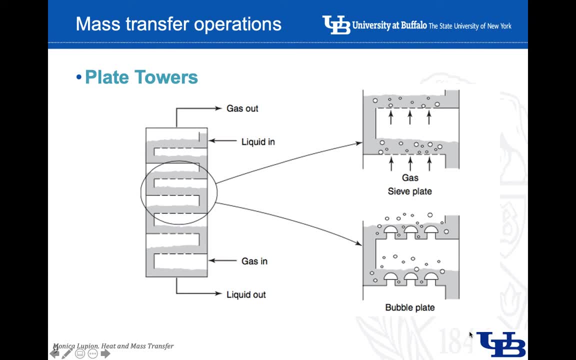 And depending on the number of trays, we can achieve better efficiency in the mass transfer operation. You see this in detail. This is a very typical example of mass transfer equipment. This is more complex, more sophisticated than the previous one, But you study how the different ratio between the liquid 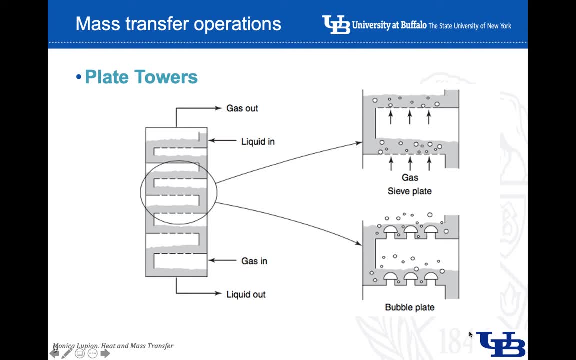 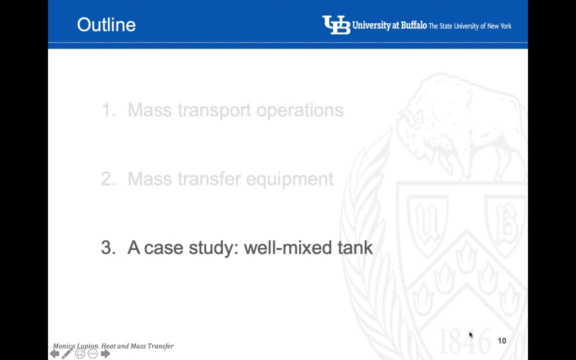 and the gas. I mean, there are different parameters that you need to take into consideration when designing a plate tower. And finally, the case study is a well-mixed tank. This is the diagram. here, What we have is a tank filled with liquid. 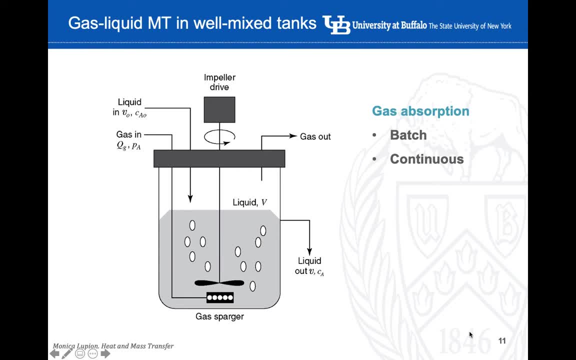 And we incorporate a gas And using a device to produce bubbles, because we know that with bubbles, what we achieve is a better contact between the phases And therefore we can achieve a better mass transfer operation. It's important as well that it's well-mixed. for the same reason, 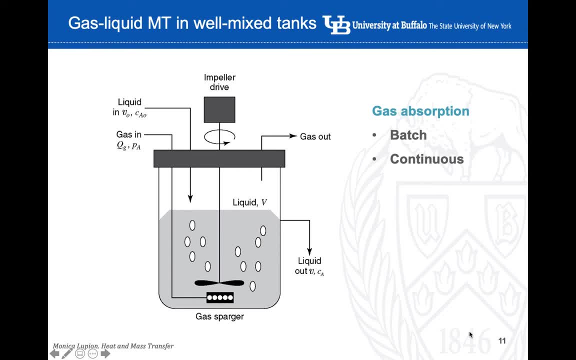 We want the mixture as homogeneous as possible In order to make the contact better. We're going to see two different examples And we're going to apply the equations that we know about mass transfer in two different situations. One is batch operation And the second case is continuous operation. 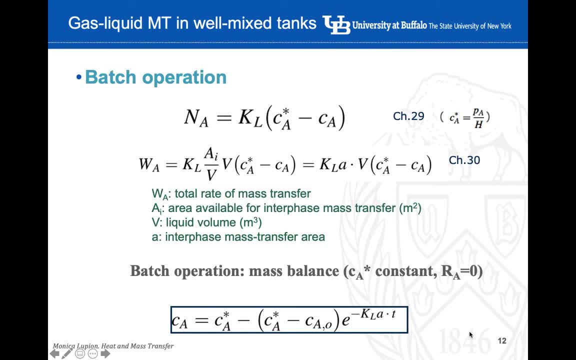 In batch operation, when we study the equations, once the- let's say, the concentration- has reached some stable number. So we are defining this batch operation when it's a steady state, So there is no dependence with time, Something that we're calling in chemical engineering. 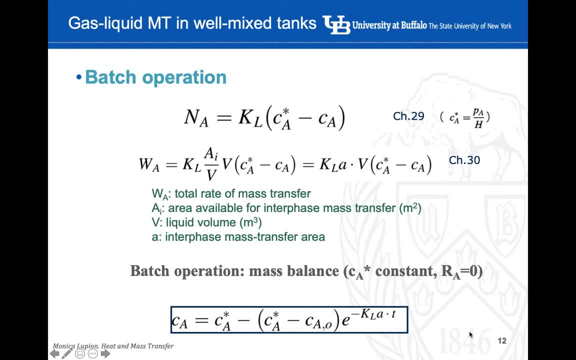 as permanent conditions. So once we reach to these stable conditions we can apply the mass transfer, the convective mass transfer equation that we know. The monoflux of A is equal to the overall convective coefficient. in the liquid times, the delta concentration. 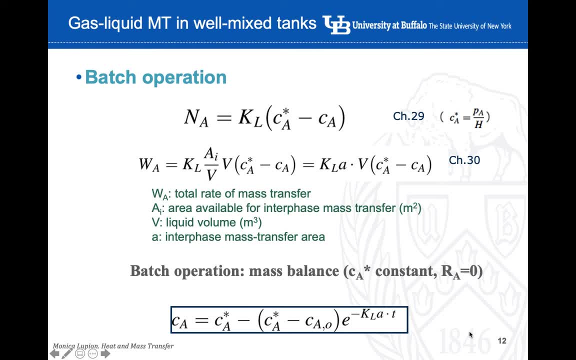 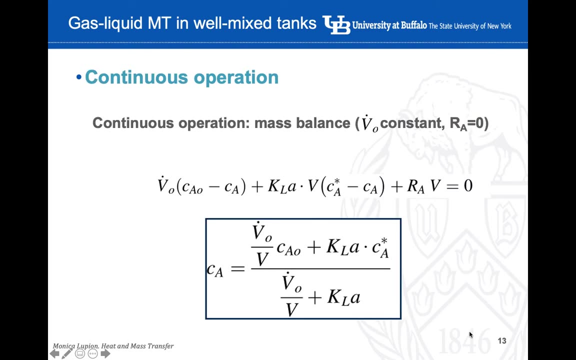 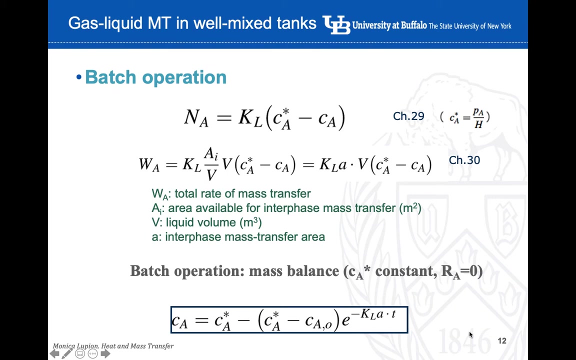 which is the driving force. Delta concentration is defined as the concentration of the element A in the equilibrium, minus the initial concentration of the element A. So with that we can define the total rate of mass transfer, just multiplying this monoflux by the interface mass transfer area A. 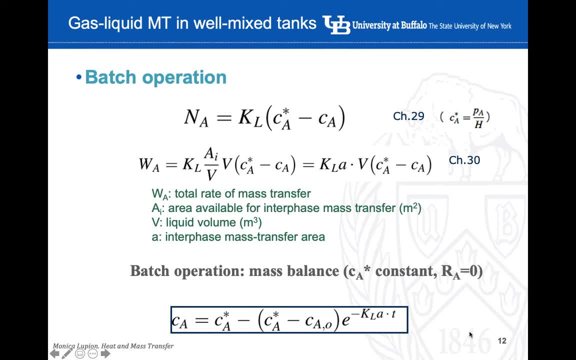 which is defined as the ratio between the area available for the interface mass transfer divided by the total area of the tower, usually in relation to the diameter and also the volume of the tank, the capability, the capacity in volume of the tank. We play around with this equation. 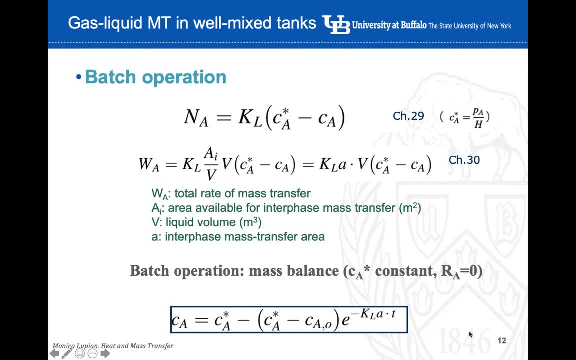 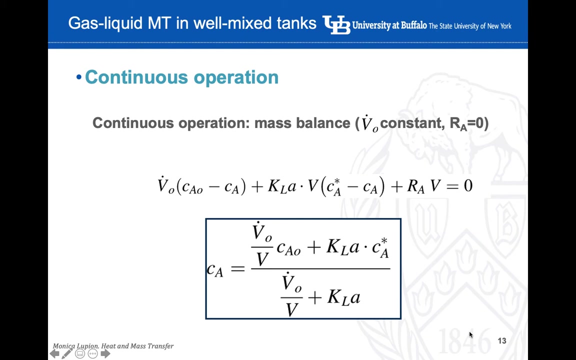 and we apply mass balance, considering that the concentration in the equilibrium is constant and also that there is no production of chemicals during the process. We play around and this is the equation that we can get boxed in black For continuous operation. the approach is a little bit different. 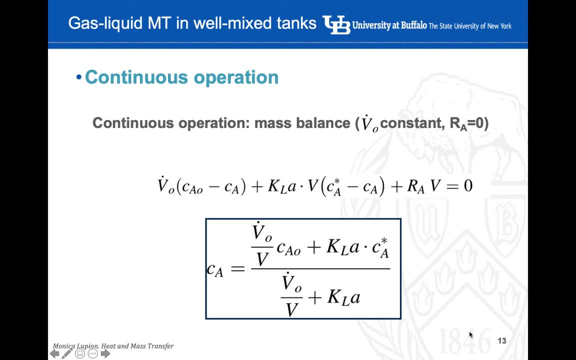 So what we do is to formulate a mass balance. So what is getting in minus what is getting out plus what is being transferred from one phase to another, plus, if there is any generation due to chemical reaction is equal to zero, We can assume that there is no chemical reaction. 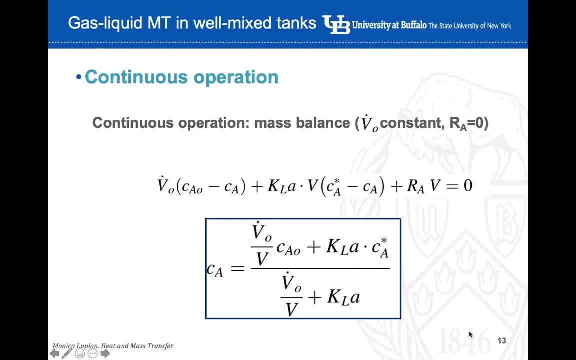 and therefore the last term, air A times volume is equal to zero. so we can cancel that. And if we want to calculate what's the concentration of the element A, we can just play around with the equation, the mass balance equation. and well, you have the definition. 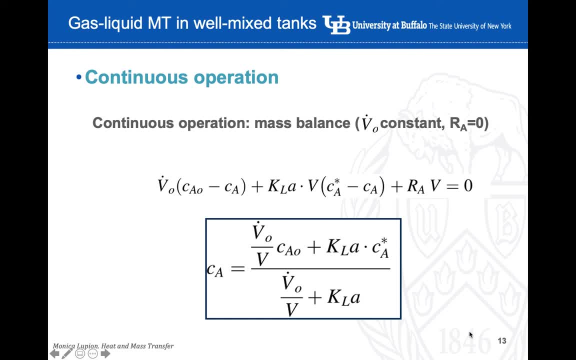 of the concentration of the element A boxed in black. What is important here is that there is a you need to know the initial concentration and as well the concentration in the equilibrium which you will have to define, taking into account the, for example, the Henry laws. 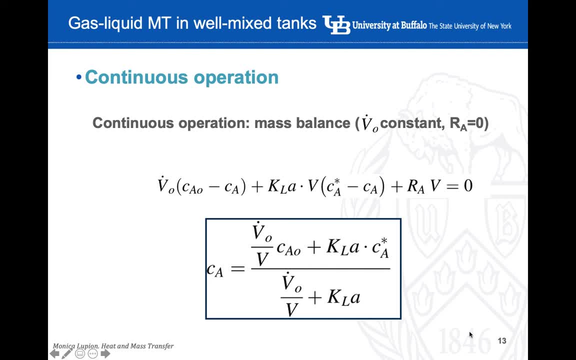 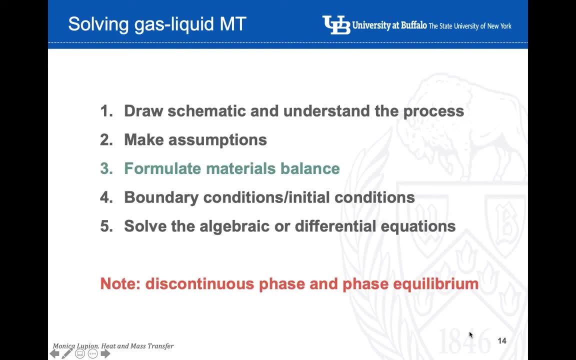 You can know the vapor pressure in the equilibrium in order to calculate this concentration of the element A. So, in general, as a summary, if- and again, this is more for the senior course, the separation course, when you find mass transfer equipment. 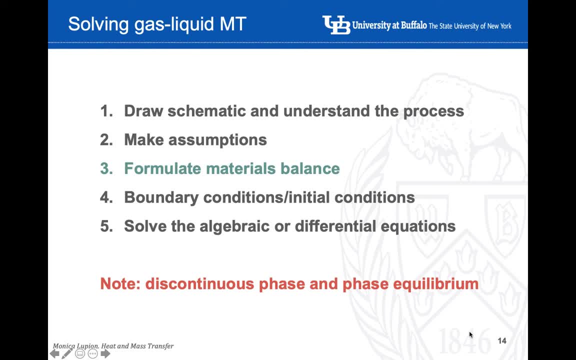 it's important, as always, that you understand how the process is, that you can understand the main elements of the equipment. So if it helps a lot if you can draw a diagram, then we make assumptions, For example, if there is no chemical generation. 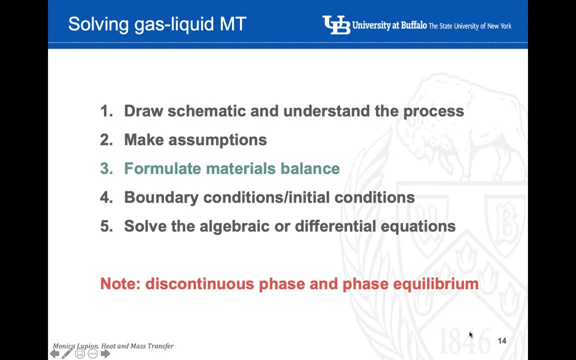 if we can consider a steady state that will help a lot to solve the equations involved, Then in all this equipment you will have to formulate the material balance, always in all of them: What is getting in, what is getting out? 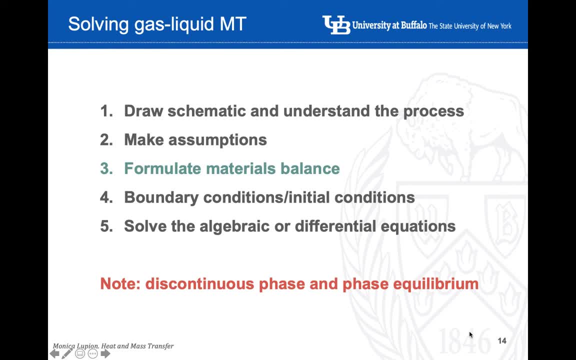 if there is an accumulation within the equipment and if there is any generation, Then to determine the boundary conditions and the initial conditions and finally to solve the equations. So it's very similar to what we've seen so far In this case.